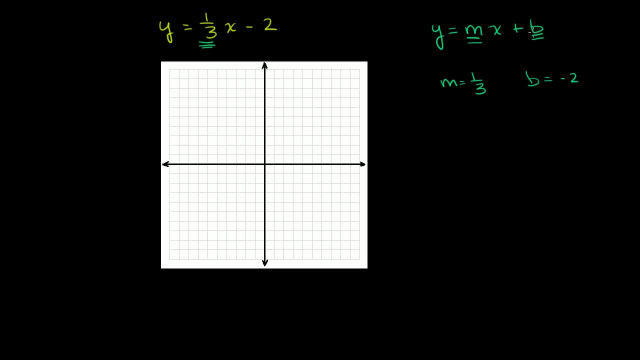 And you know that b is the y-intercept, because we know that the y-intercept occurs when x is equal to 0. So if x is equal to 0, in either of these situations, this term just becomes 0, and y will be equal to b. 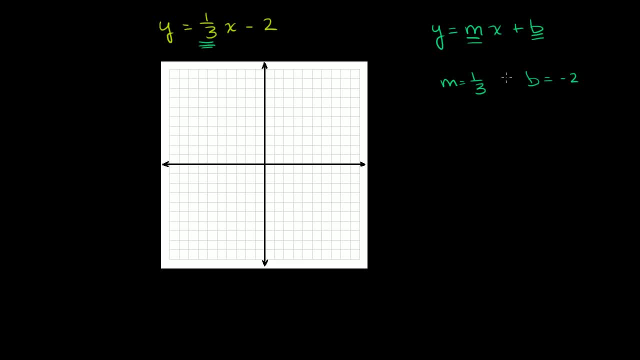 So that's what we mean by b is the y-intercept. So whenever you look at an equation in this form, it's actually fairly straightforward to graph this line: b is the y-intercept. In this case it is negative 2.. 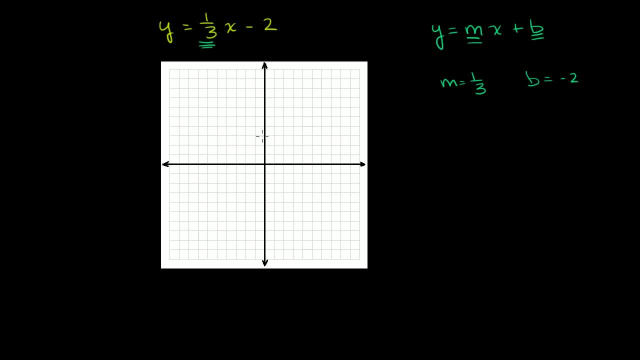 So that means that this line must intersect the y-axis at. y is equal to negative 2.. So it's this point right here: Negative 1, negative 2.. This is the point: 0, negative 2.. If you don't believe me, there's nothing. 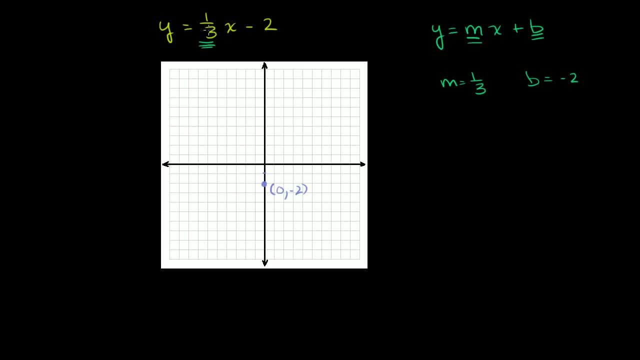 magical about this. Try evaluating or try solving for y when x is equal to 0.. When x is equal to 0, this term cancels out and you're just left with y is equal to negative 2.. So that's the y-intercept, right there. 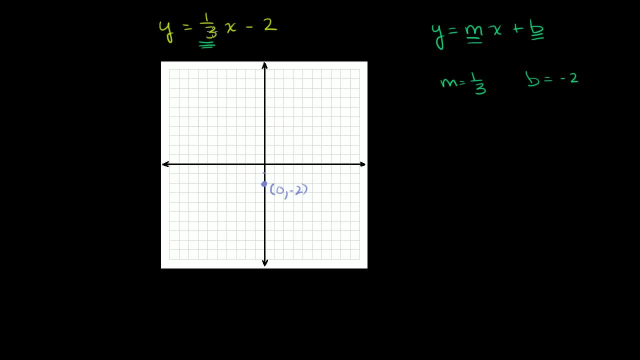 Now this 1 third tells us the slope, the slope of the line. How much do we change in y for any change in x? So this tells us that 1 third, so that right there is the slope. so it tells us that 1 third is equal to the change in. 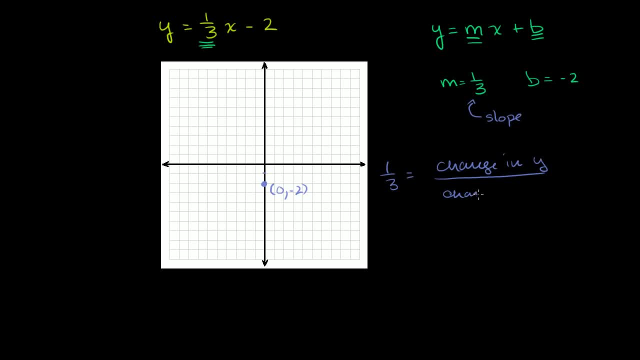 y over the change in x, Or another way to think about it. if you're going to write a graph and you're going to think about it, if x changes by 3, then y will change by 1.. So let me graph that. 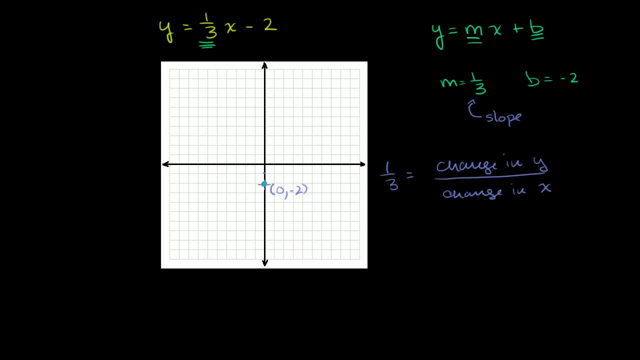 So we know that this point is on the graph. That's the y-intercept. The slope tells us that if x changes by 3, so let me go 3 to the right, 1,, 2,, 3, that y will change by 1.. 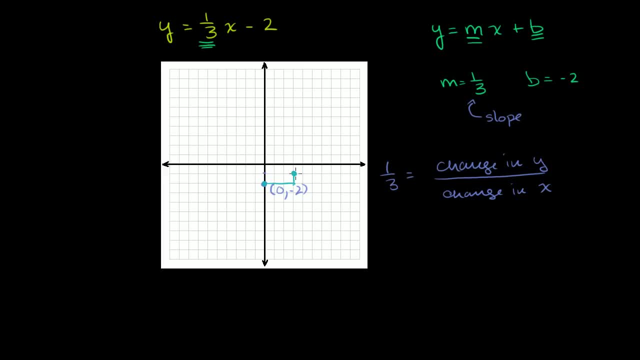 So this must also be a point on the graph, And we could keep doing that. If x changes by 3, y changes by 1.. If x goes down by 3, y will go down by 1.. If x goes down by 6, y will go down by 2..